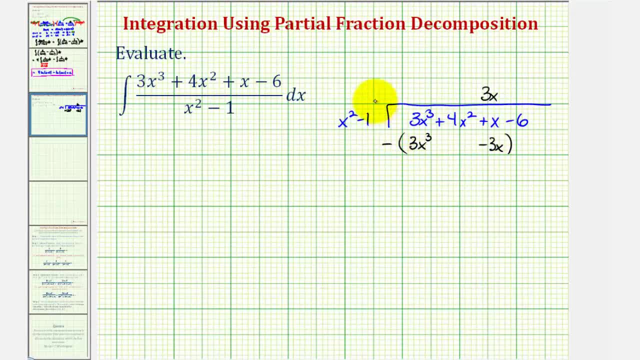 we're actually going to add the opposite instead. So we can change this to addition, as long as we change the sign of the two terms inside the parentheses. So if I change this to plus, this would be negative and this would become plus. So notice how, now. so now when we add instead of subtracting. 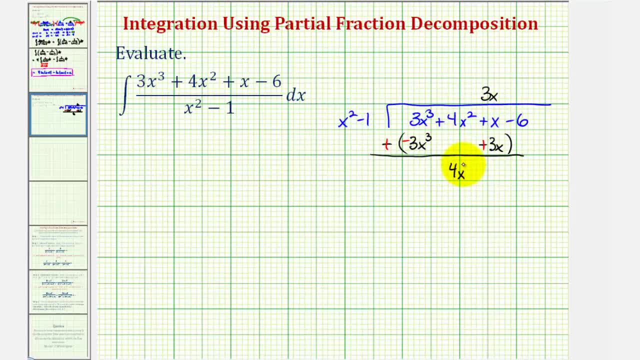 In fact, let's go ahead and bring down the four x squared. The x term would be four x. Let's also bring down the minus six. And now for the next term in the quotient, we want to determine what times x squared would give us four x squared. 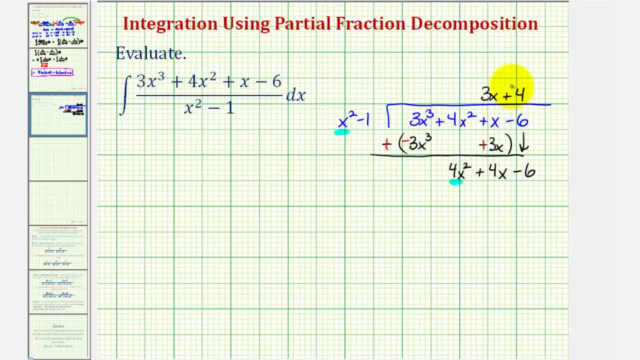 And that would be positive four. So the next term is plus four. And now again we're going to multiply this term in the quotient and the divisor. So four times x squared is four. x squared, Four times negative one would be minus four. 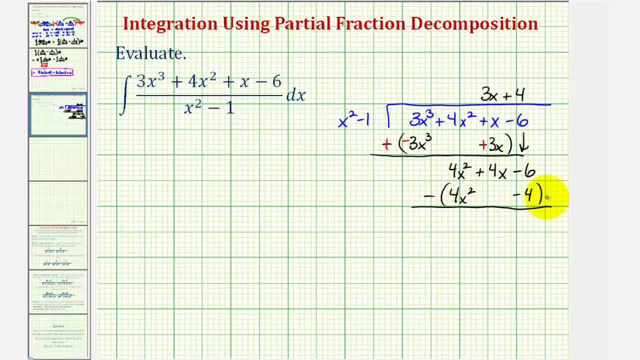 Again, we'll subtract by adding the opposite instead. So we'll change the sign here to plus. change the sign here and change the sign here. Notice, when we add down, we bring the four x down and this would be minus two. 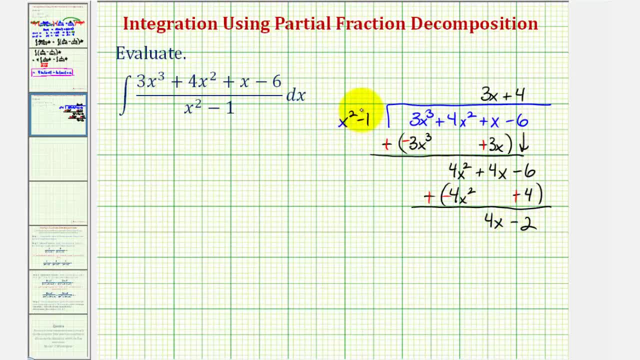 It's okay to have a degree one remainder, because our divisor is degree two. So what we've discovered so far is this integral can be written as the integral of three x plus four, plus a remainder which we'll write as the quantity four x minus two. 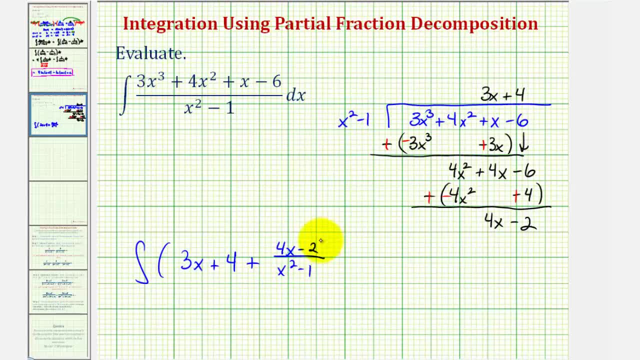 divided by the quantity x squared minus one. So now we can easily integrate the first two terms. but we're still left with this rational expression. So again we might try u-substitution by letting u equal x squared minus one, and then differential u would be two x, d, x. 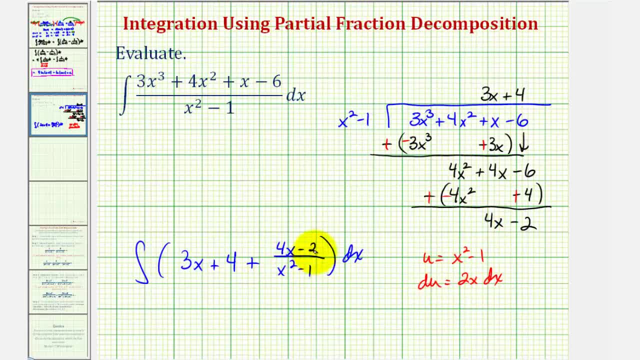 And so, while we could actually use this substitution if we broke this fraction up into two separate fractions, meaning we could write this as four x divided by the quantity x squared minus one, minus two divided by the quantity x squared minus one. So this u-substitution would help us integrate. 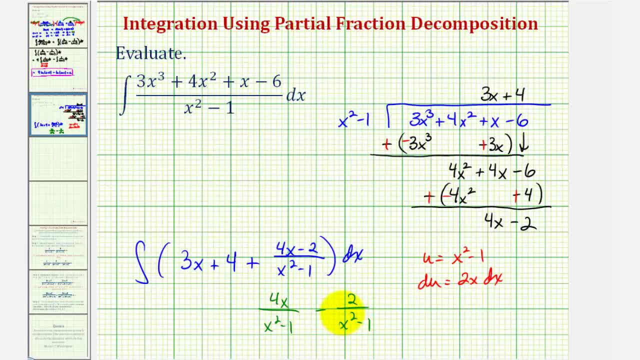 this part here, but not this second fraction. So what we're going to do is go ahead and leave it in this form here and then perform partial fraction decomposition on this rational expression. So let's go ahead and do that on the next slide. 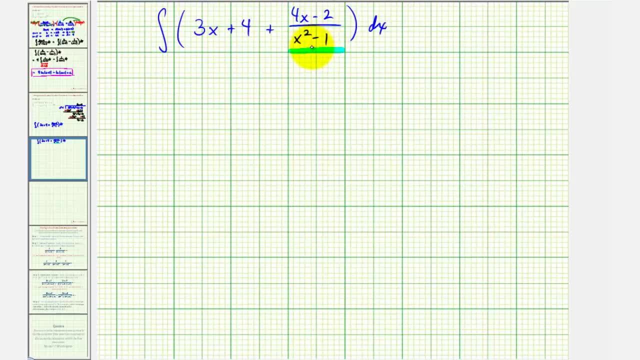 So now we're just going to take this rational expression here and write it as the sum or difference of fractions. that will hopefully be easier to integrate. So to begin, let's rewrite this and factor the denominator, So we would have the quantity four x minus two. 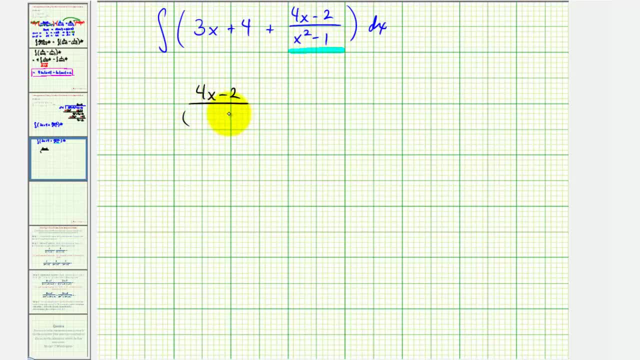 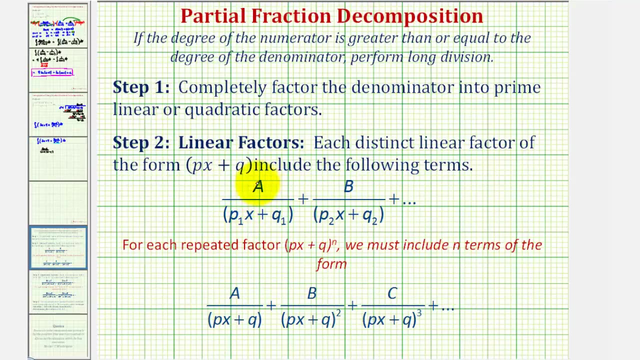 divided by this is a difference of squares, so we have x plus one times the quantity x minus one. And because our denominator contains two distinct linear factors, we're going to write this as a sum of two separate fractions, where we'll have a constant. 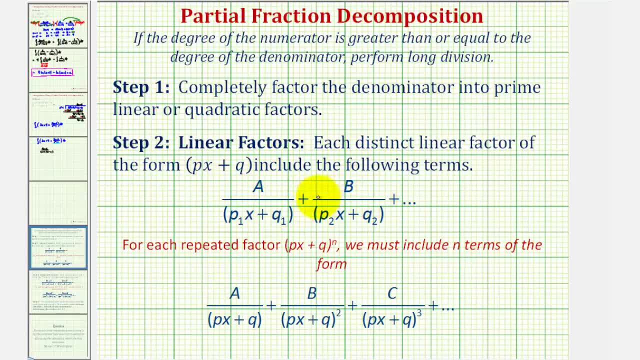 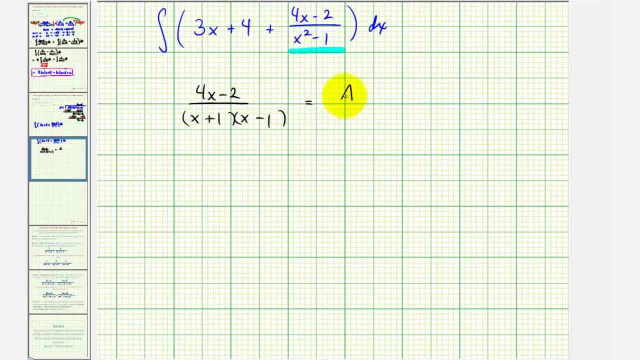 divided by the first linear factor plus a constant divided by the second linear factor, Meaning we'll have a divided by the second linear factor divided by the quantity x plus one plus b times the quantity x minus one. So once we determine the values of a and b, 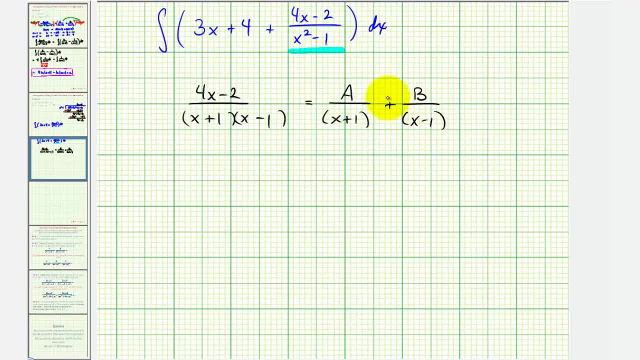 we can rewrite this rational expression as this sum. So for the next step, we're going to clear the denominators from this equation by multiplying both sides of the equation by the least common denominator, which would be the quantity x plus one times the quantity x minus one. 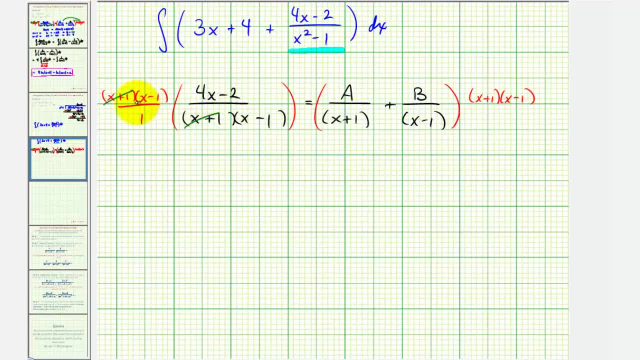 Notice on the left side: x plus one over x plus one and x minus one over x minus one simplify out, leaving us with just four x minus two equals on the right side. notice in this first product: here one factor of x plus one simplifies out. 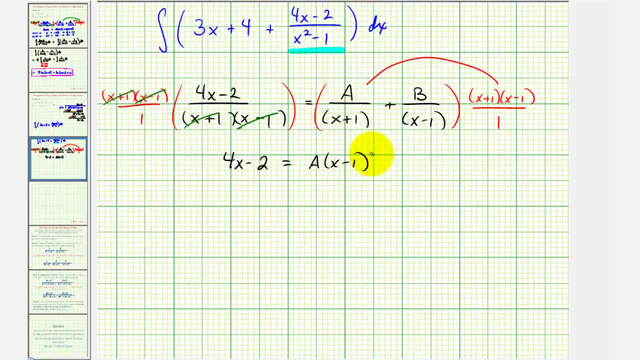 leaving us with a times the quantity x minus one. And then for this second product, here, one factor of x minus one simplifies out, leaving us with plus b times the quantity x plus one. This is called the basic equation which we now want to solve for a and b. 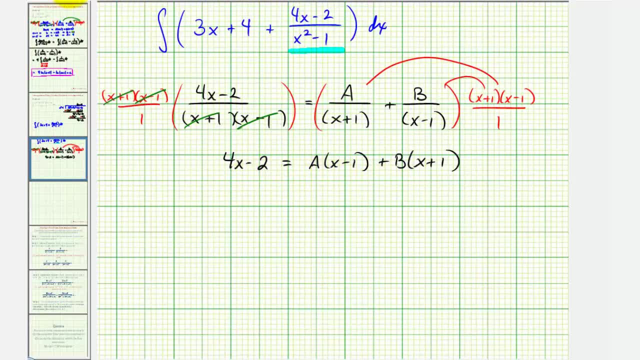 by selecting convenient values of x. For example, notice: if we let x equal positive one, this product here would be zero. So if x equals one, we'll substitute one for x. that would be four minus two or two equals. 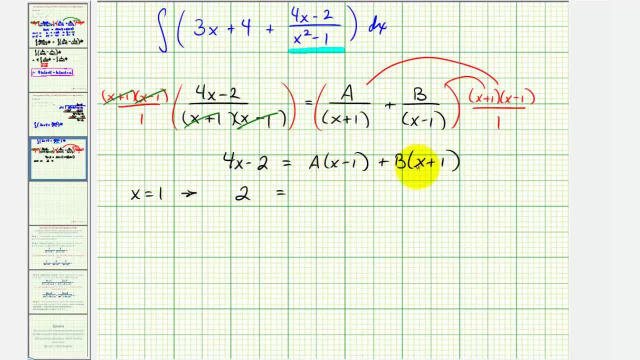 again, if x is one, this would be zero plus b times the quantity one plus one or two b Notice: here we can determine that b equals one. and now to determine the value of a, we'll select: x equals negative one. 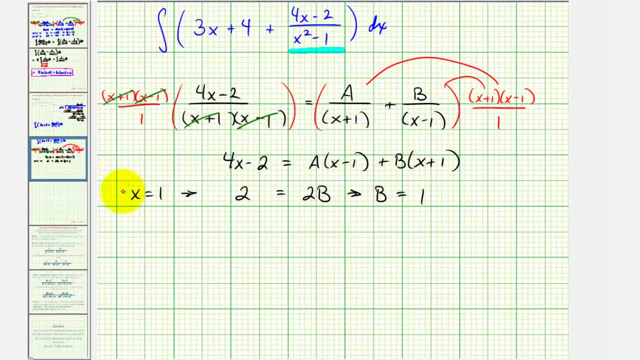 which would make this factor zero and therefore this product zero. So if x equals negative one, this would be negative four minus two, that's negative six equals this would be a times negative two or negative two a, and again this would be zero. 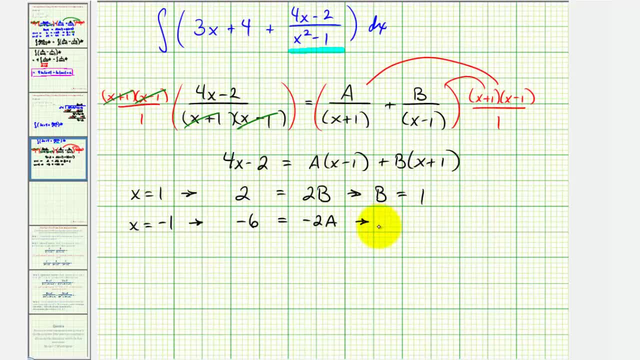 Notice how here, if we divide both sides by negative two, we can determine that a equals three. So now, if we substitute one for b and three for a, we can rewrite this rational expression as this sum. So we can write this integral here. 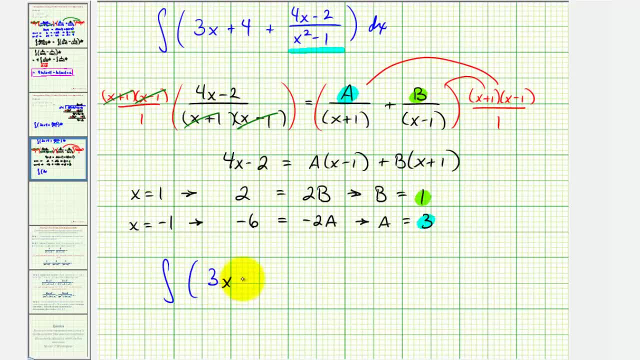 as the integral of three x plus four plus. since a is equal to three, we would have three divided by the quantity x plus plus since b is one, we'd have one divided by the quantity x minus one. So again, the whole point of doing this is: 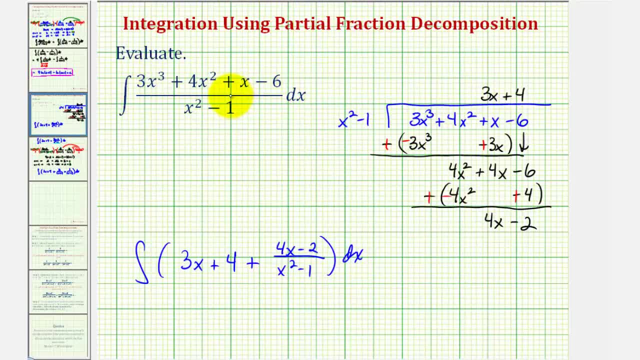 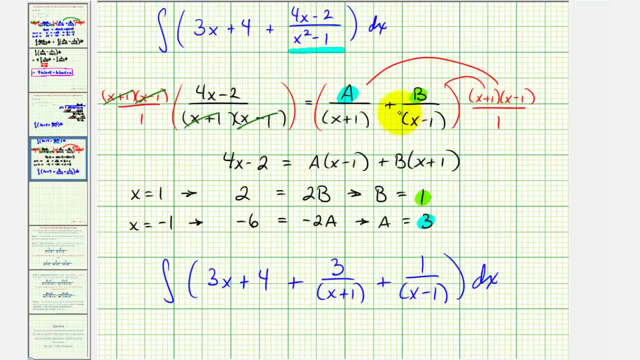 going back to the original integral. we weren't able to integrate this in its current form, so we performed long division and then, to help us integrate this piece here, we performed partial fraction decomposition, which gave us the sum of these two rational expressions: 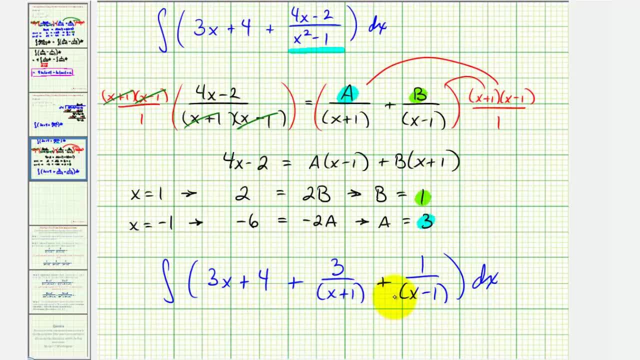 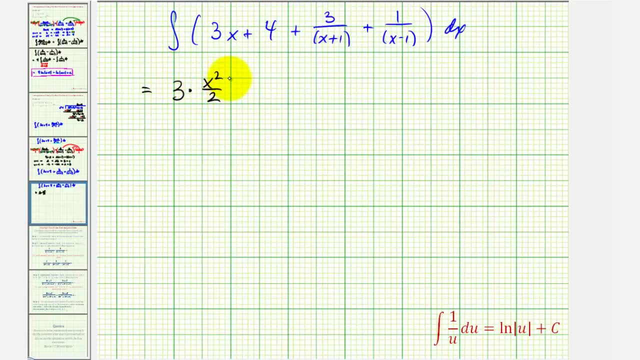 and hopefully now, in this form, we can now integrate. Let's go ahead and do this on the next slide. The antiderivative of three x would be three times x to the second, divided by two, plus the antiderivative of four would just be four x. 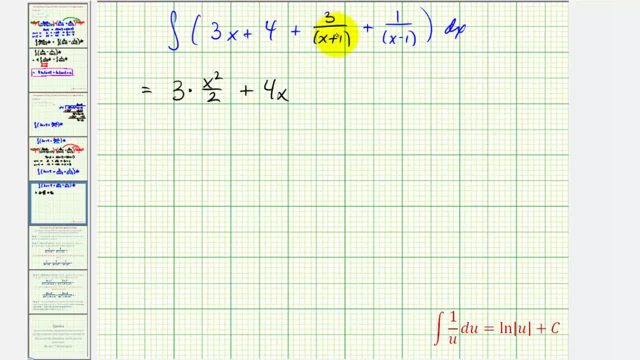 To find this antiderivative, we might be thinking we need to perform u-substitution. but notice, if u is equal to x plus one, then differential u would just be equal to dx. So this fits the form of the integral of one over u du.